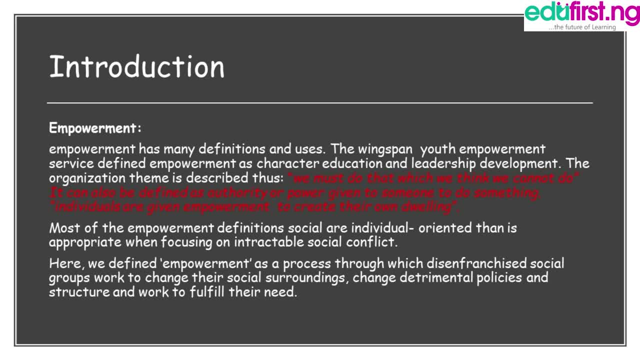 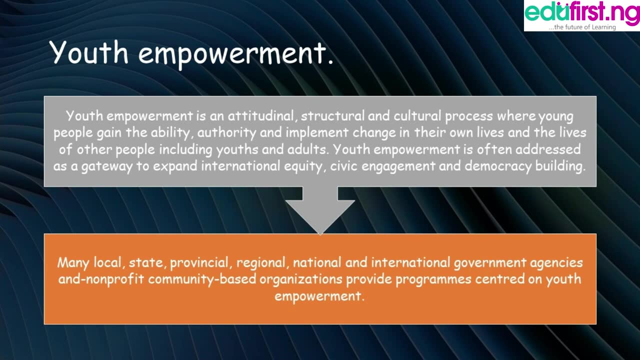 Here, however, we defined empowerment as a process through which different sized social group work to change their social surroundings, change the policy and structure, and work to. DEAR is an actuarial, structural and cultural process where young people gain the ability, authority and implement change in their own life and the life of other people, including. 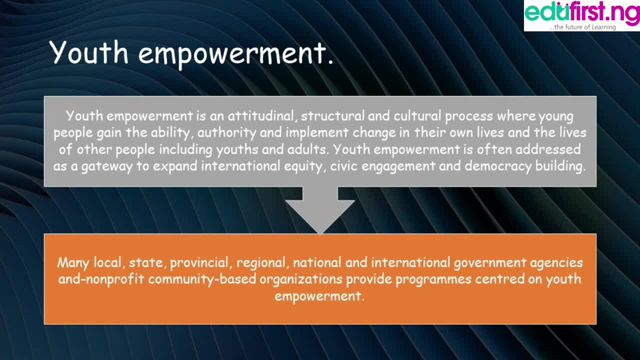 youths and adults. Youth empowerment is of time, addressed as a gateway to expand international equity, civic engagement and democracy building. Many local, state, province, regional, national and international government agencies and non-profit community-based organizations provide programs, tools and resources for youth empowerment. 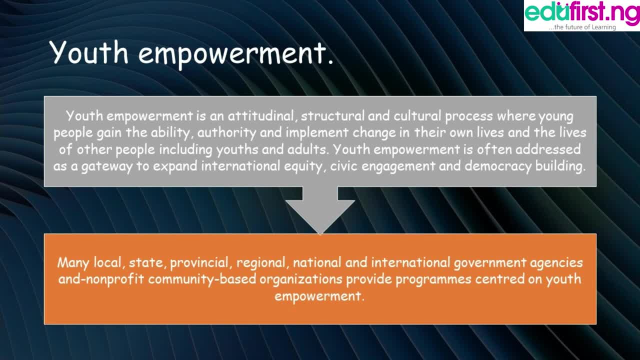 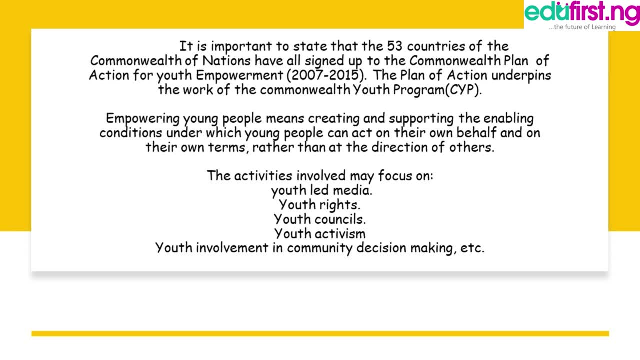 center on youth empowerment. It is important to state that the 53 countries of the Commonwealth of Nations has all signed up to the Commonwealth Plan of Action for Youth Empowerment In 2017 to 2015,. the Commonwealth Plan of Action for Youth Empowerment was adopted by 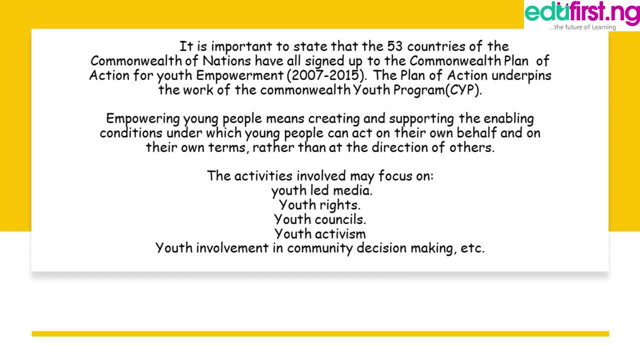 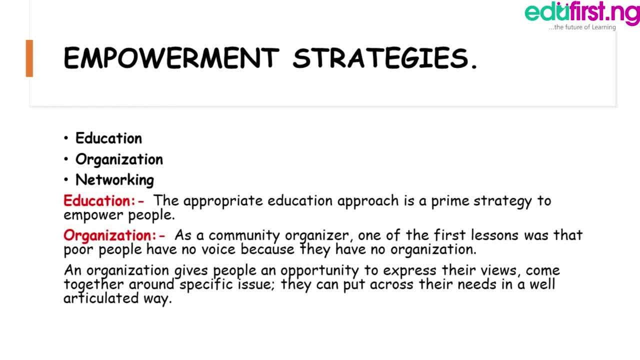 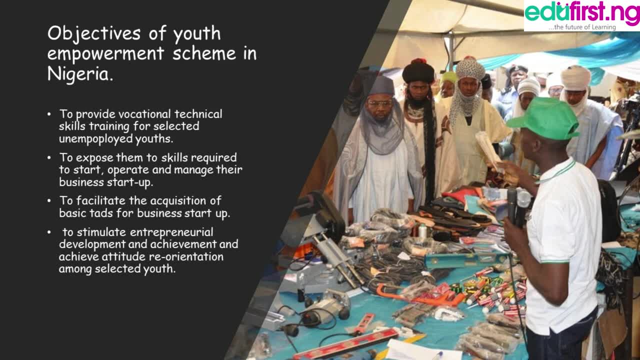 into other people's websites. Objectives of Youth Empowerment Scheme in Nigeria. The objective, the motive of this Youth Empowerment Scheme in Nigeria is to provide vocational technical skills training for selected unemployed youths to expose them to skills required to start, operate and manage their own business set-up. 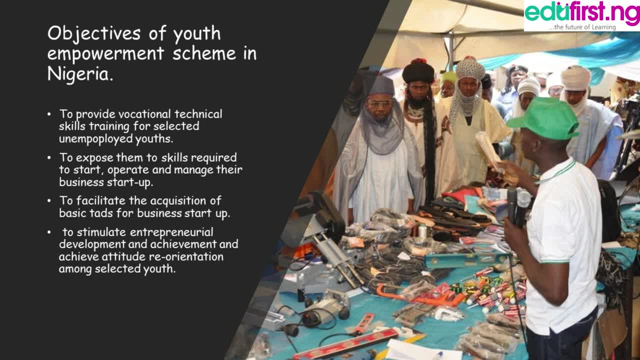 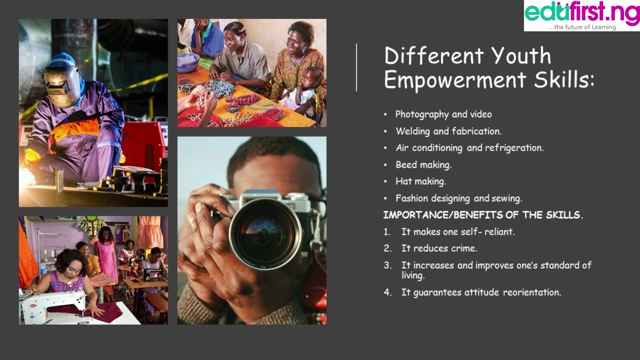 The third objective is to facilitate the acquisition of basic things, of business set-up, to stimulate entrepreneur development and achievement and to achieve attitude reorientation among selected youth. We have different types of Youth Empowerment Scheme. We have the Photographers, we have the Video, we have the Wedding and Fabrication, Air Conditioning. 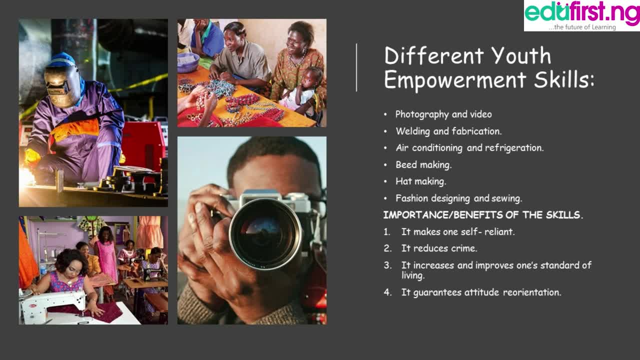 and Refrigeration, Bead Making, Hat Making, Fashion Designer and Sewing. The importance or benefits of these skills are number one. it makes one self-reliant. it reduces the burden of self-reliance. It reduces the burden of self-reliance. 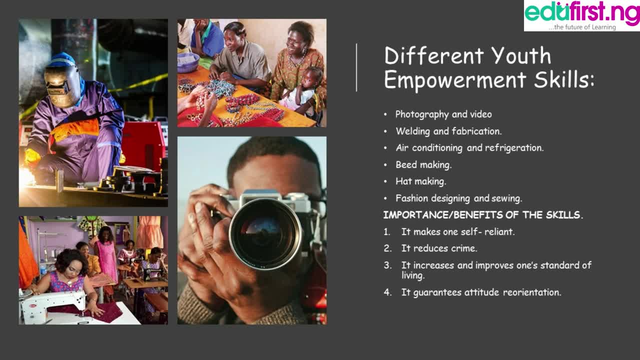 It reduces the burden of self-reliance. It increases the stability of the youth community and the quality of life of people. It increases the awareness of the youth community and the knowledge of the people. It reduces the burden of self-reliance. 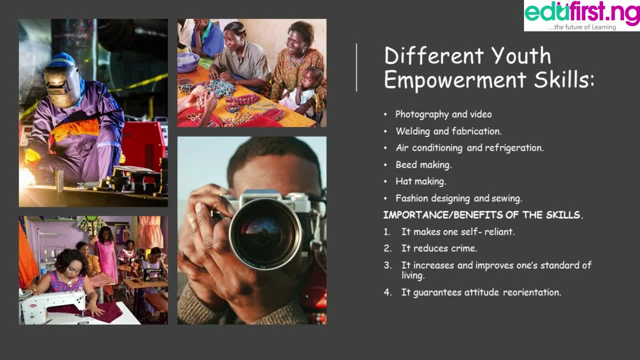 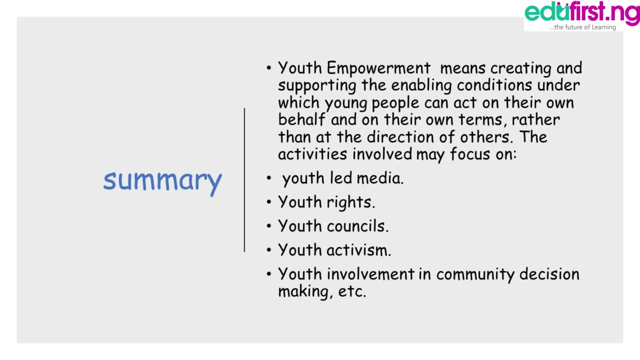 It reduces the burden of self-reliance. It increases the burden of self-reliance and improves one's standard of living. It generates attitude reorientation. In summary, Youth Empowerment means creating and supporting the enabling condition under which young people can act on their own behalf and on their own terms, rather than at the 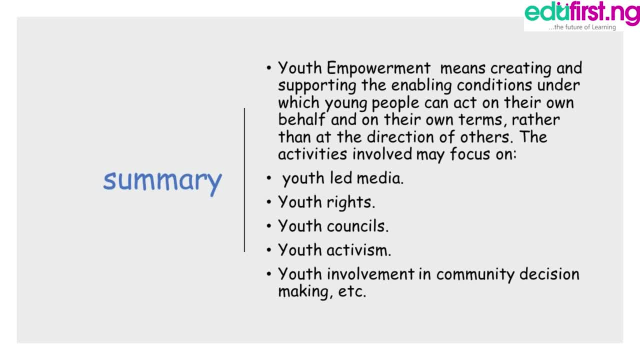 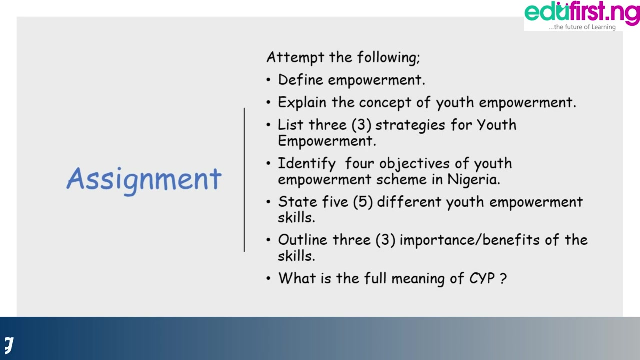 than at the direction of order. the activity involved may focus on youth led media, youth rights, youth cancer and youth autism. youth involvement in community decision making. before we leave, let's take assignments. i think the following defines empowerment: discuss two empowerment strategies, you know. identify four objectives of the youth.